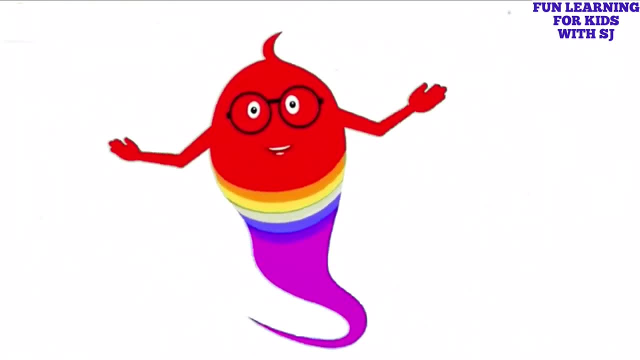 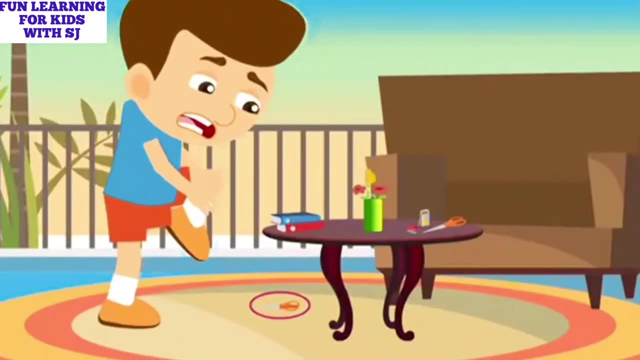 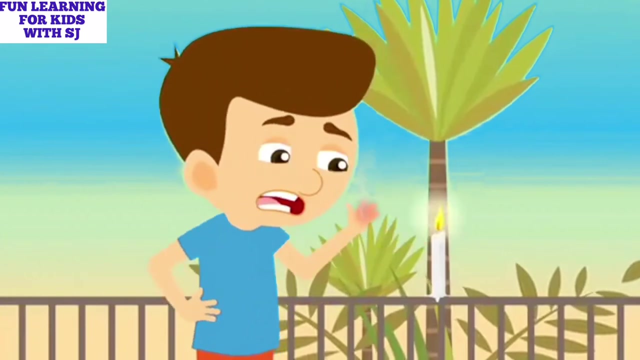 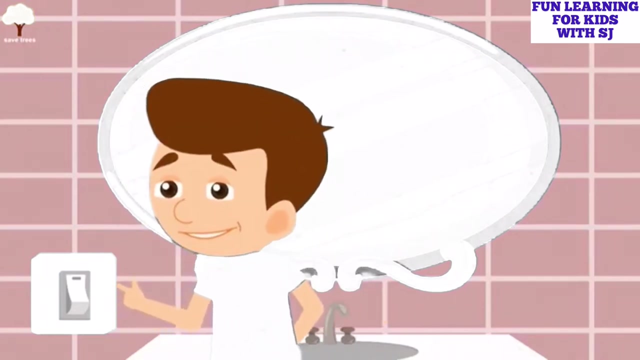 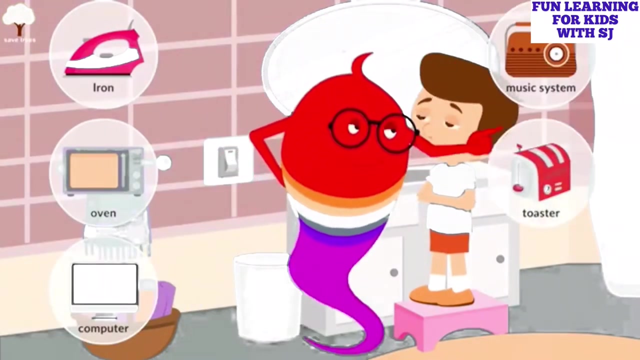 These can be extremely harmful for us. For example, if you play with scissors you might get cut, And playing with fire is dangerous: You may burn yourself or your house might catch fire. Do not touch electrical equipment like switches and wires, Hot irons, oven, computer music system, toasters and other electric items with wet hands. 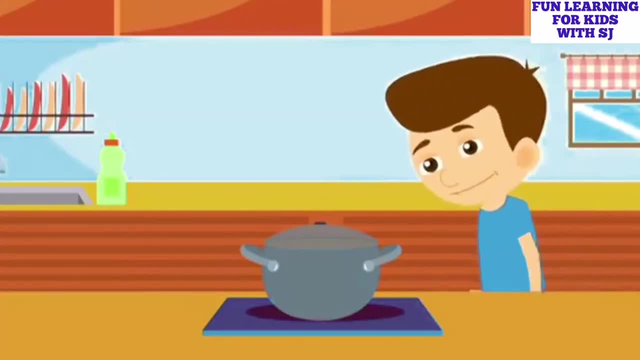 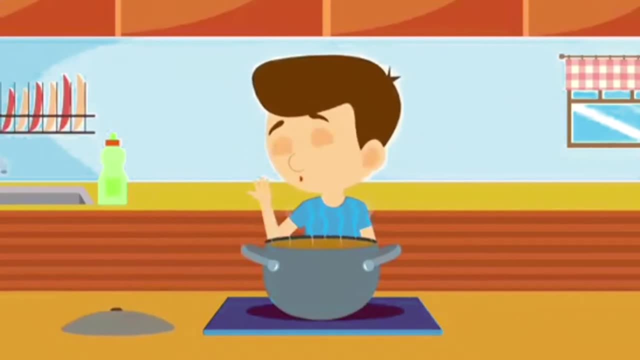 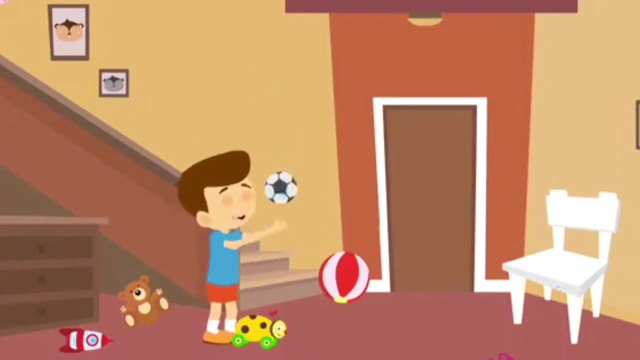 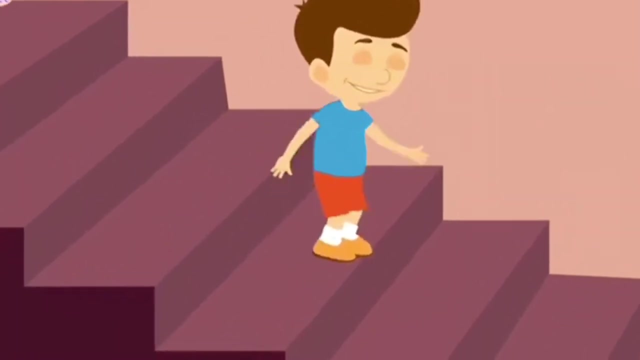 It may give you an electric shock. Do not go near the stove or touch the hot pans. You may burn yourself. Keep your toys, bags and other items in the proper place. You, or anyone else, should be careful. Do not push anyone or run and jump on the stairs. 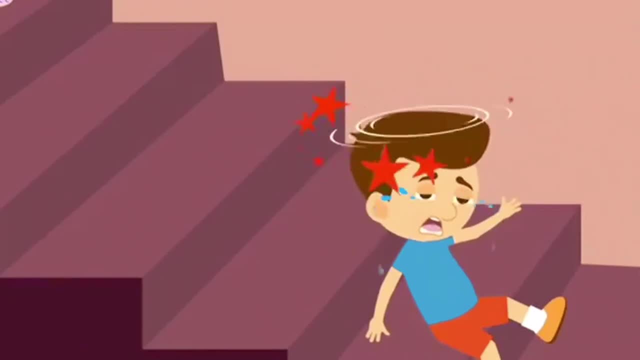 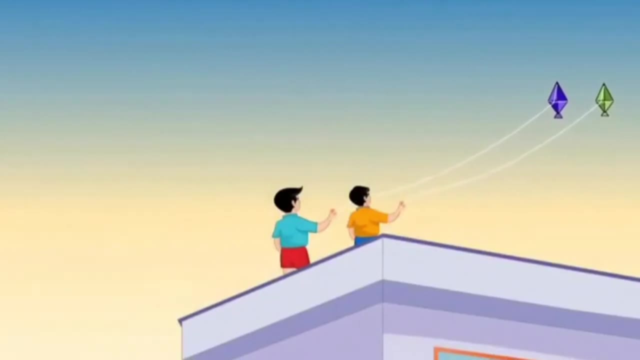 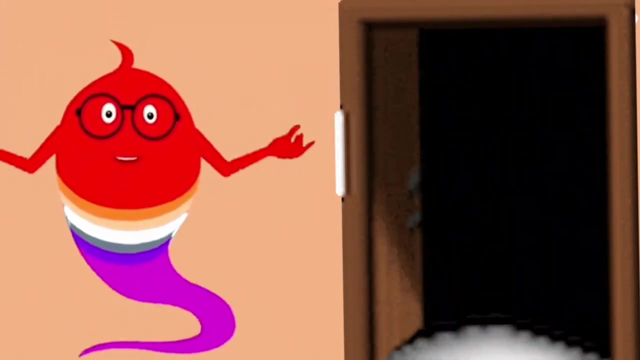 You may hurt yourself or others. Do not fly kites on the roof of your house. Go to a playground to fly the kite. Be careful. Never open the door for strangers. They may harm you, While most of the time you should be careful. 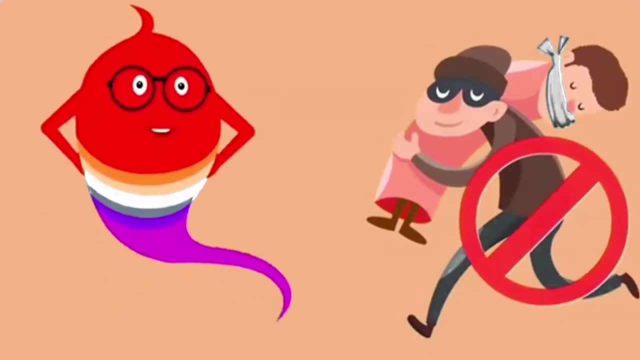 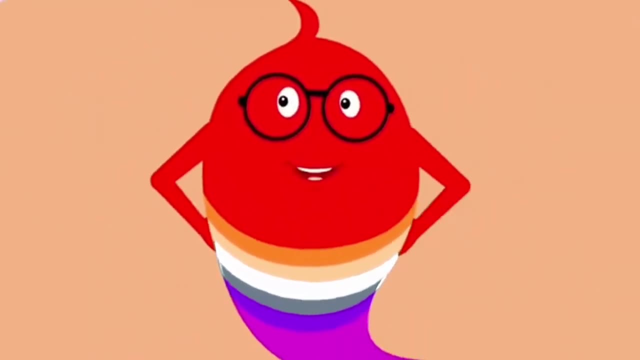 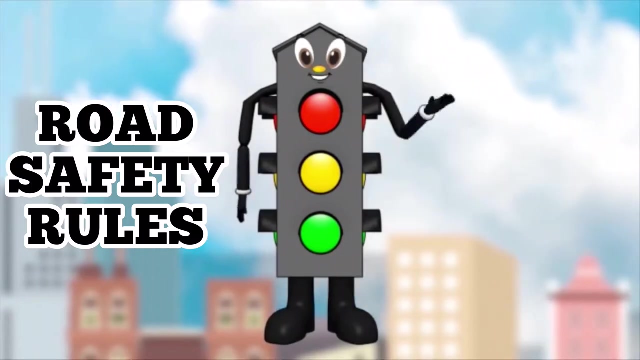 Be careful. Most people are good, but there are some bad people also who do not keep kids safe. Don't be tempted by people you don't know. Now let's see some road safety rules we should always follow. Road safety is the protection and prevention of road accidents. by using all the road safety, 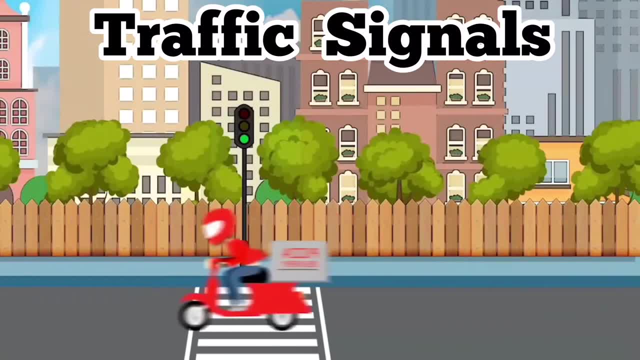 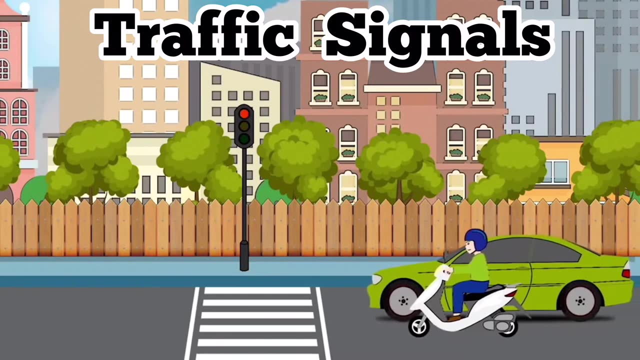 measures. Look closely. It's very important to know the traffic signals Yellow. Yellow means to slow down. When the signal turns yellow, vehicles should slow down. Red means stop. When the signal turns red, all the vehicles have to stop. 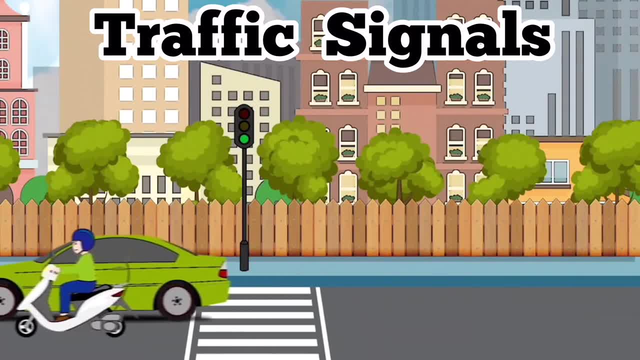 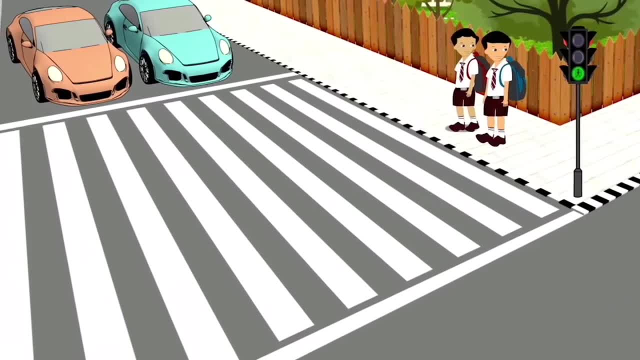 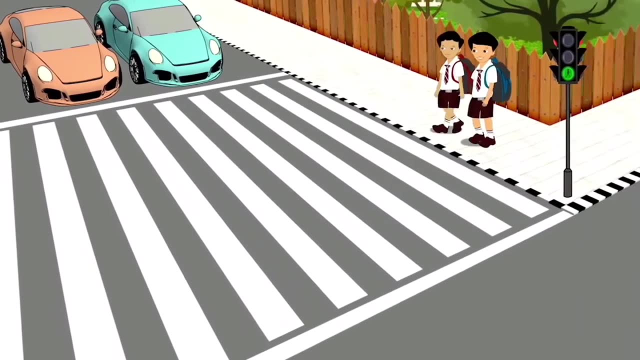 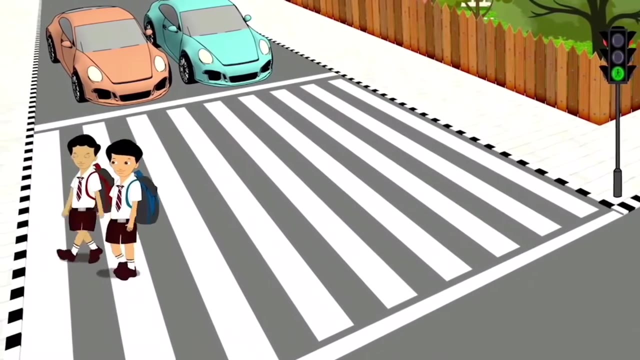 Green means go fast. Only when the signal turns green vehicles move ahead. Look both ways while crossing a street. Never cross if vehicles are coming. Use the zebra crossing only when you see the vehicles are stopped. Wear a helmet when riding a two-wheeler. 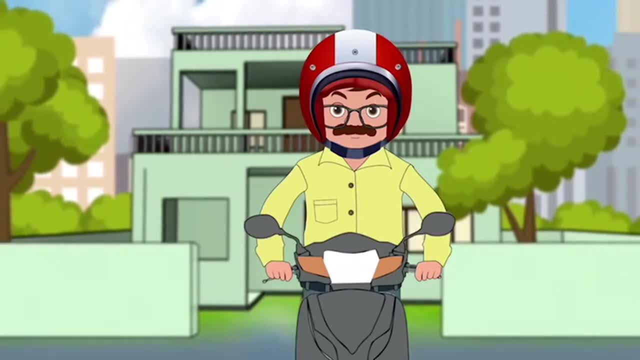 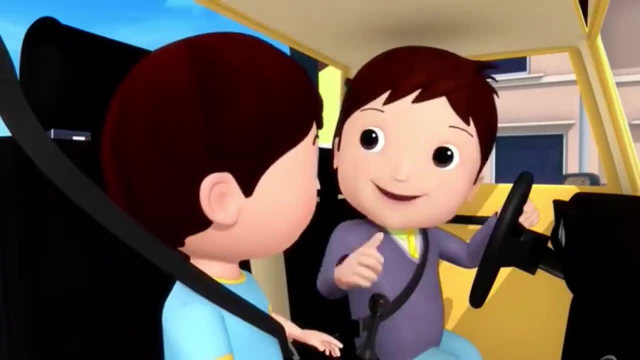 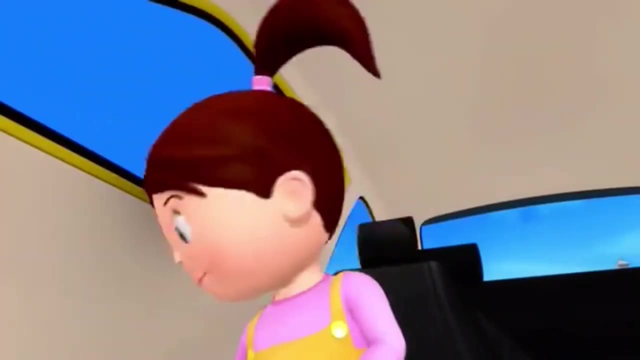 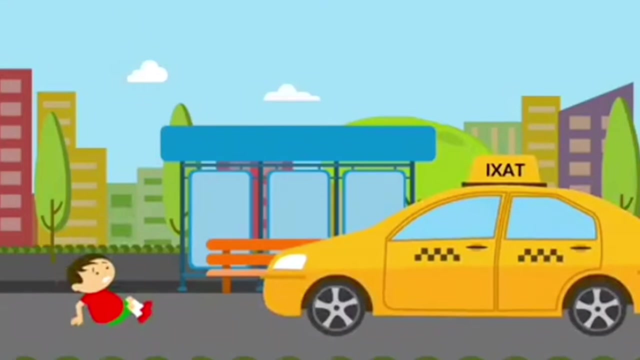 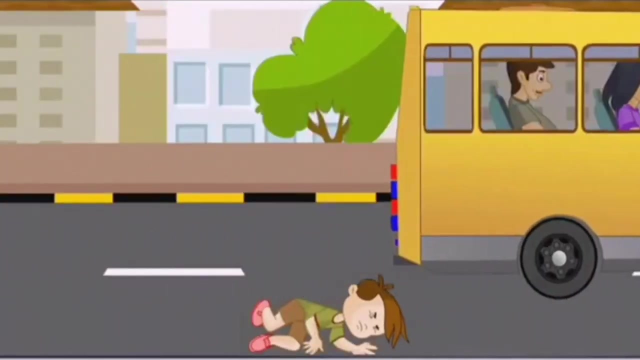 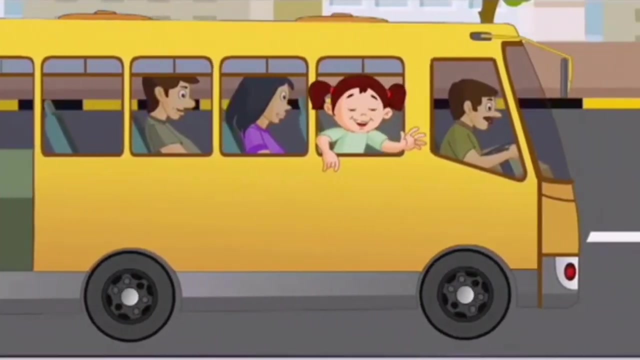 It protects us from injury. Wear a seatbelt while in the car. It helps against harmful movements like a sudden break. Don't run and play on roads. It may lead to serious accident bus You may hurt yourself. Never stick hands outside the vehicle. Some passing vehicle. 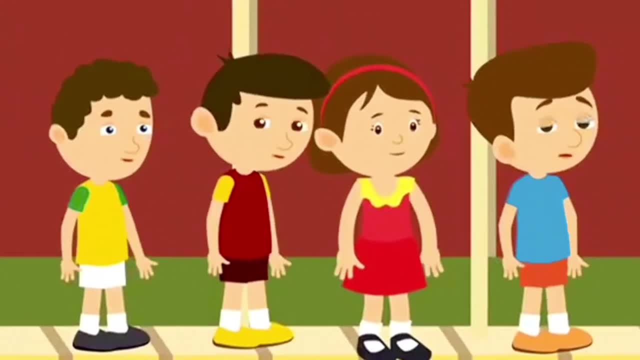 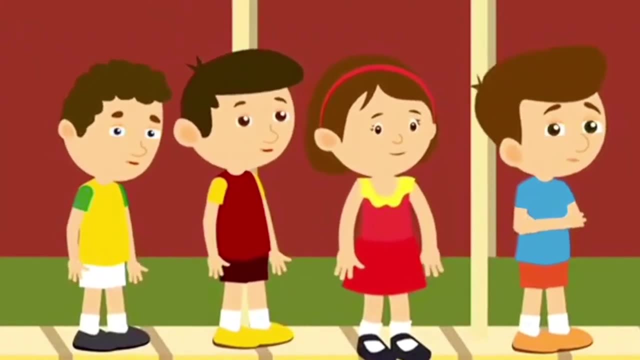 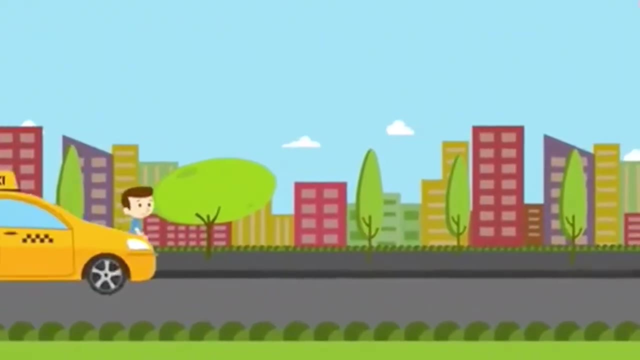 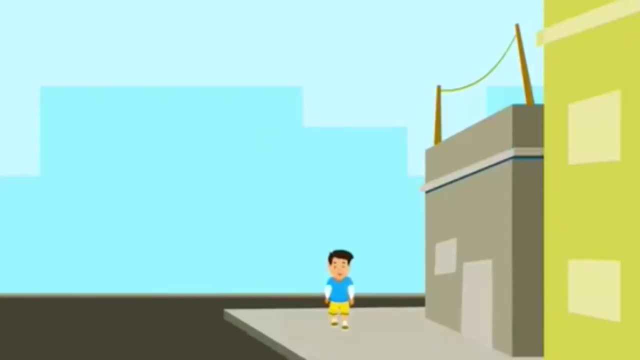 can harm you. Always stand in a queue at the bus stop while waiting for the bus. Do not push anyone. Never talk to the driver when he is driving. It is always recommended to use the sidewalks or footpath to walk. Now we will learn some safety tips for school. 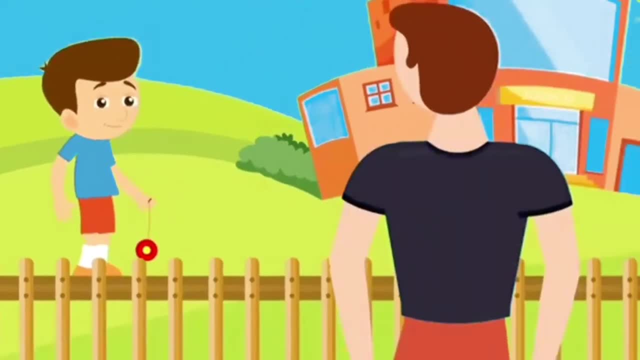 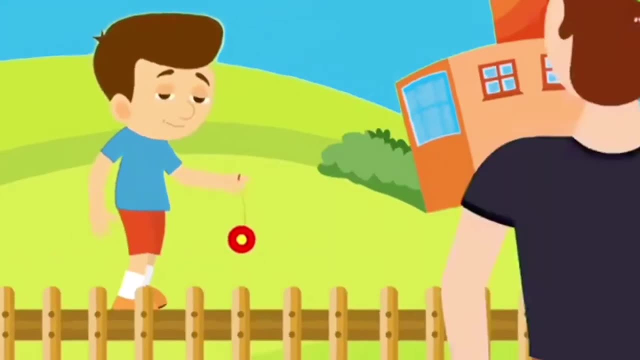 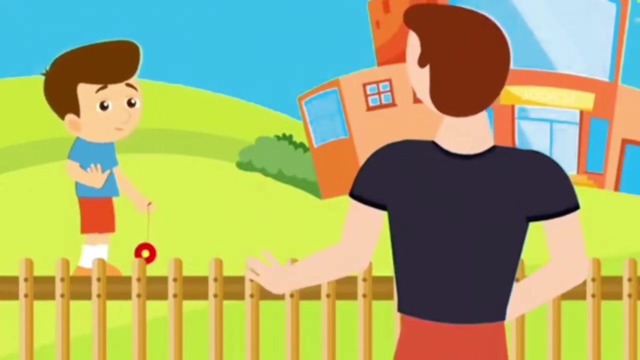 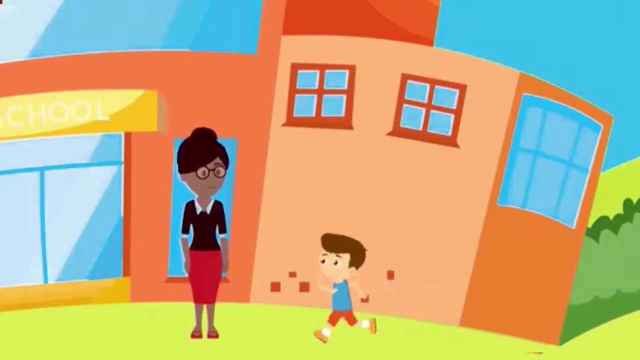 and outside. Do not ever leave your school or go anywhere with a stranger. Do not eat anything given to you by a stranger. It may be harmful for you. Do not share your secrets and family details with strangers. In case of danger, always shout for help. 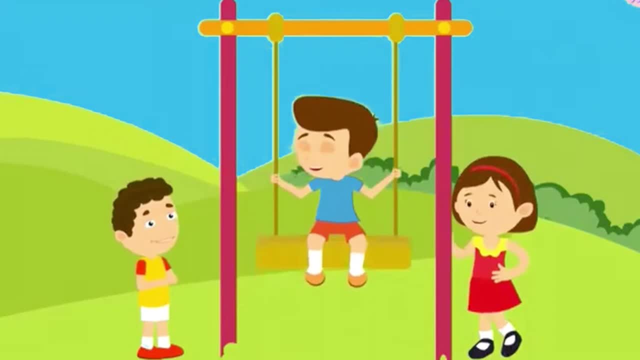 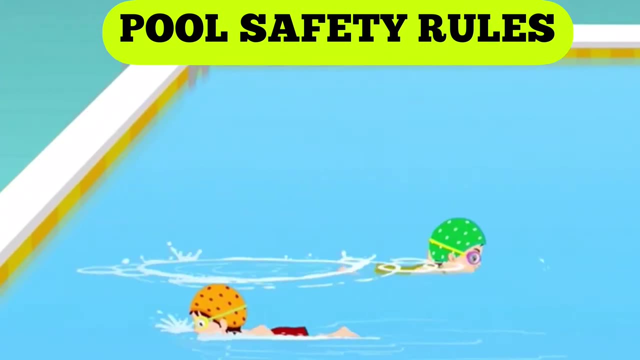 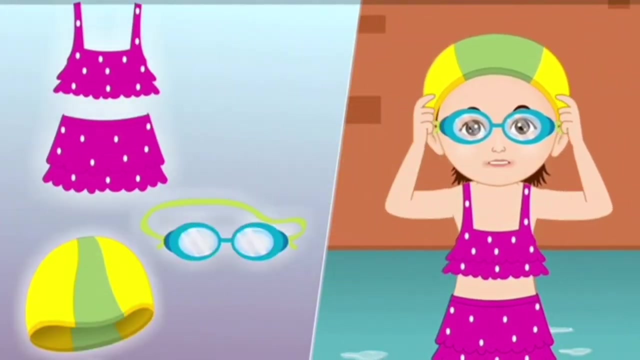 When you are on the playground, always wait for your turn on the swings. You should follow few rules at the swimming pool. Let's look at it. You should wear proper swimwear, goggles and caps while swimming. You should wear rubber shoes so that you don't. 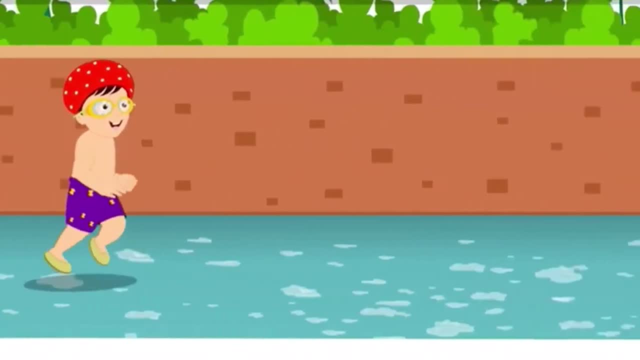 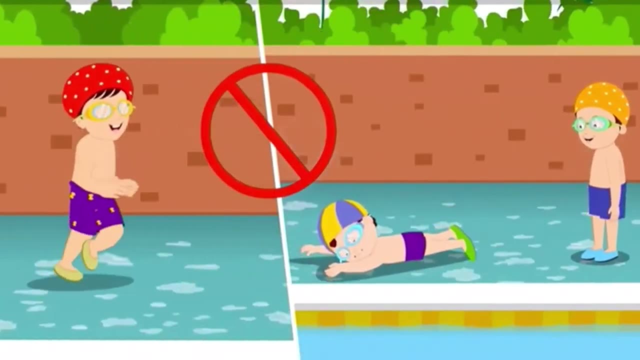 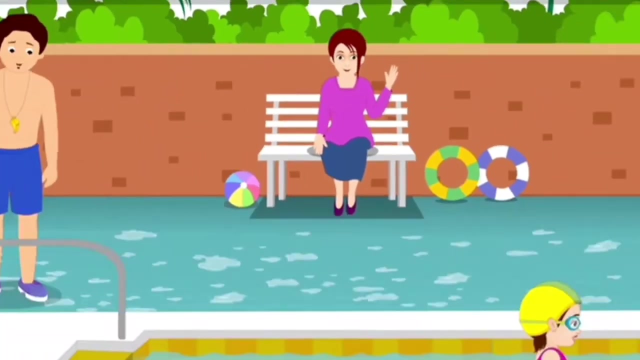 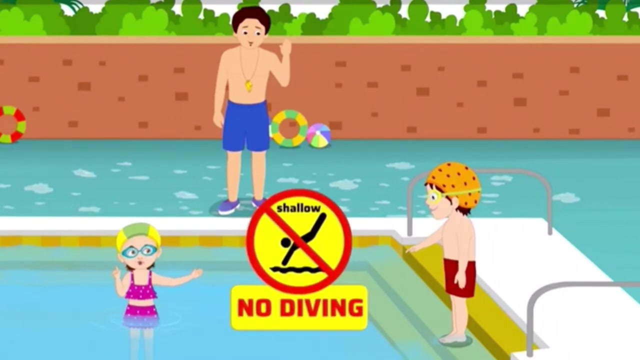 slip on the deck. the floor around the pool is usually wet, so you should never run there. you should also never push anyone. you should swim when the lifeguard is around or an adult is there with you. don't fool around or jump into the pool. if you don't know how to swim, we must use a swimming tube while 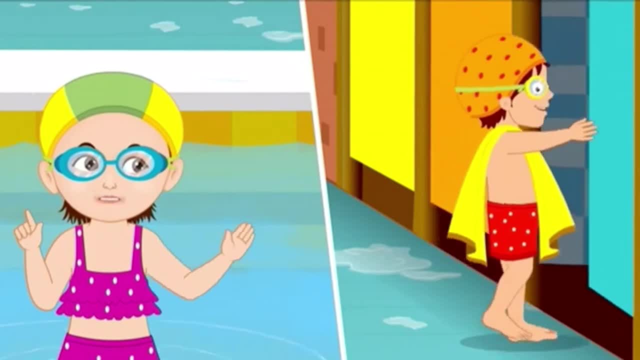 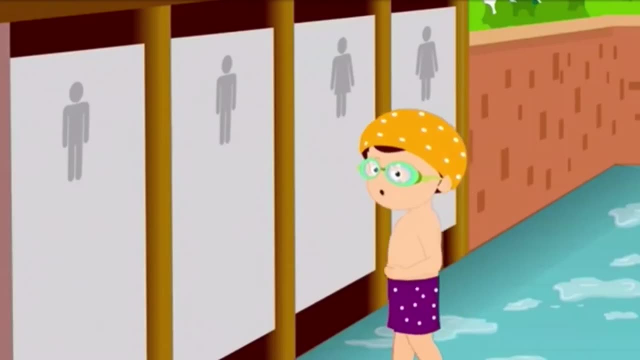 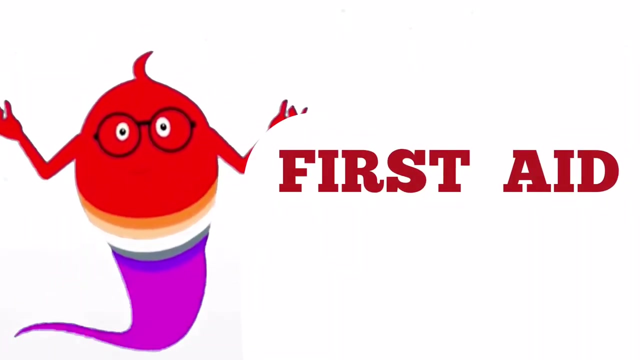 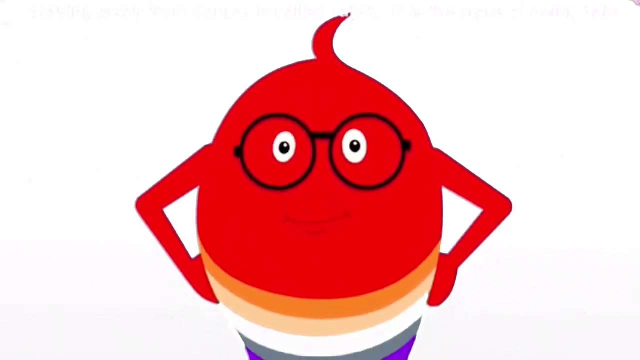 learning to swim. don't forget to shower before and after a swim. go to the restroom when nature calls you. very good. now we'll learn about something very important: first aid friends. even if we carefully follow the safety rules, we may sometimes get hurt if someone else is injured. 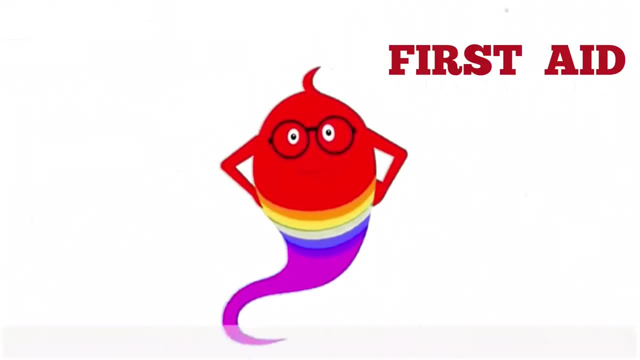 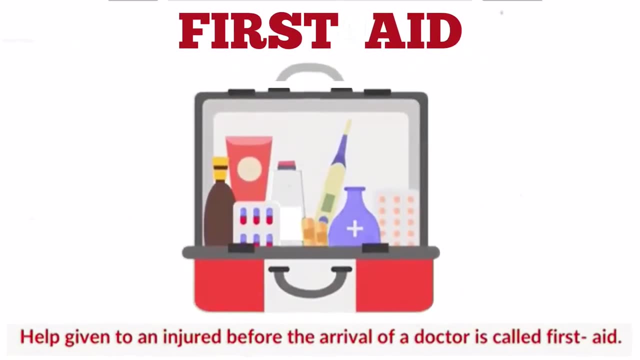 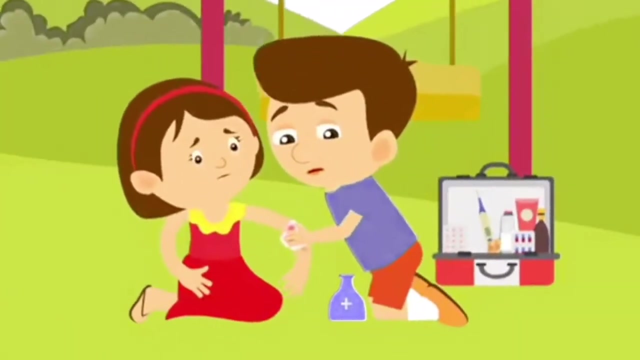 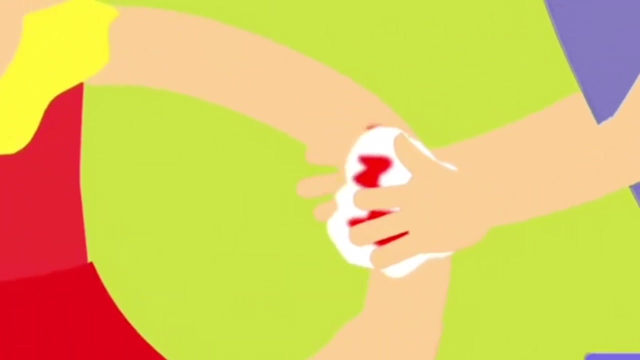 we should help them. the help given to an injured person before the arrival of a doctor is called first aid. the purpose of first aid is to minimize the injury and future disability. if someone is injured, then in case of wounds or cuts, clean it properly and then use an antiseptic lotion if an adult is there. 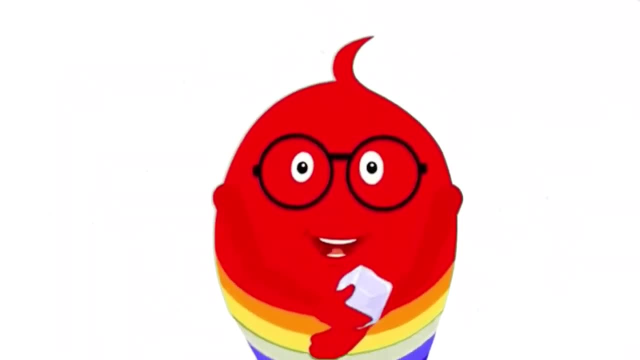 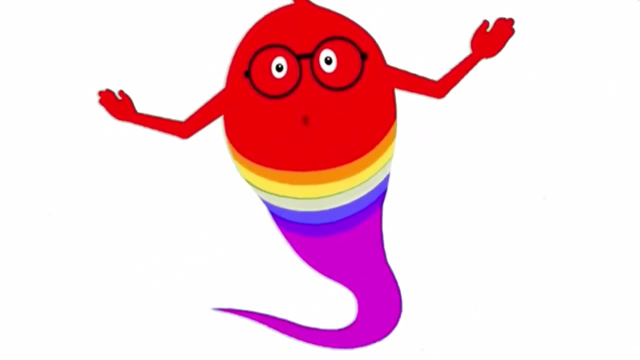 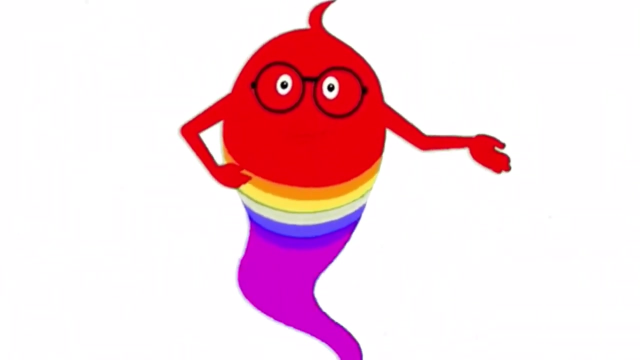 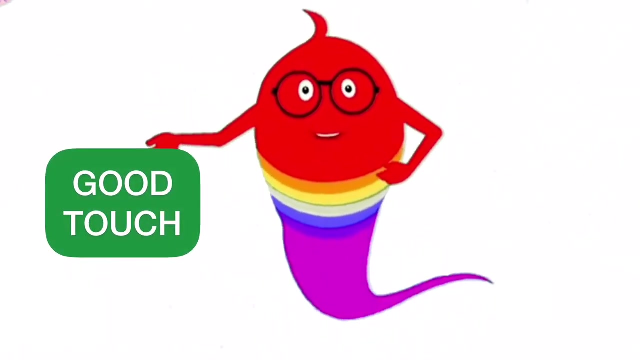 help. if there's a minor burn, ice cubes can be applied for relief. if it's a major accident and no one is around, immediately dial the emergency number. friends, now it's time to learn something that is most important: good touch and bad touch, friends, when mama goes to the bathroom and she doesn't want to go to the bathroom. 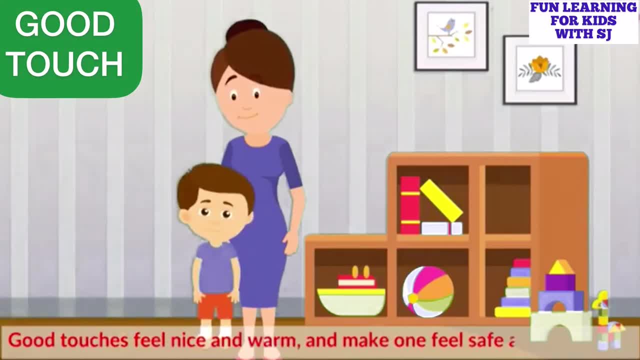 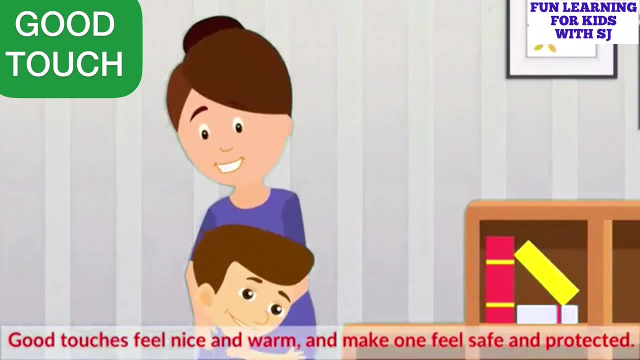 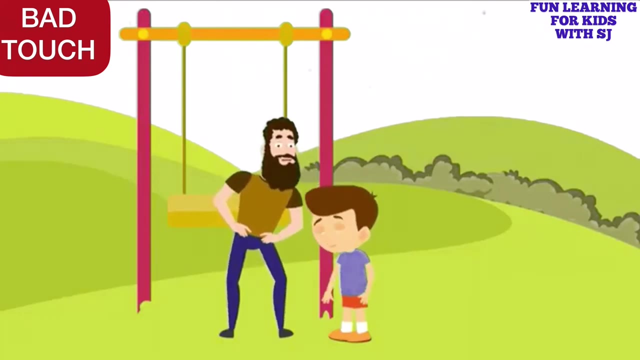 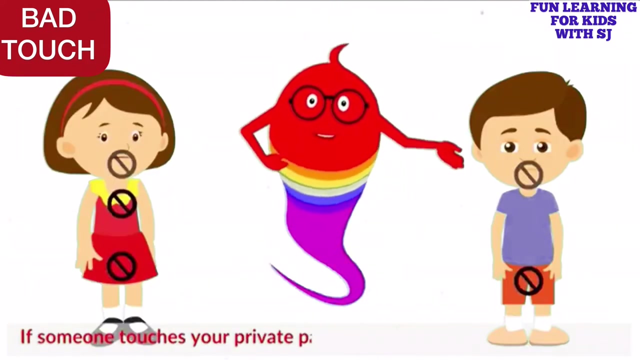 gives you a hug or daddy gives you a goodnight kiss, it makes you feel happy, comfortable and safe. it is good touch. but sometimes, when a person touches you and you get an uncomfortable feeling, it's bad touch. if someone touches your private parts without a reason, it's a bad touch. 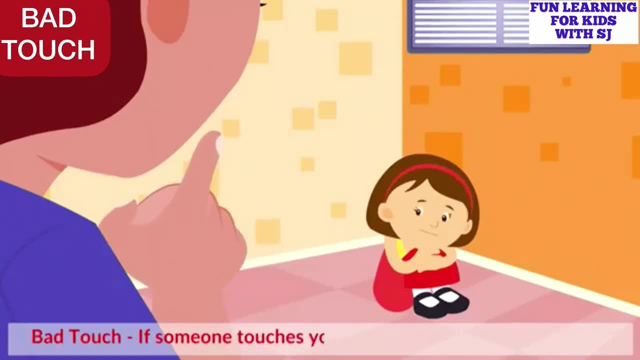 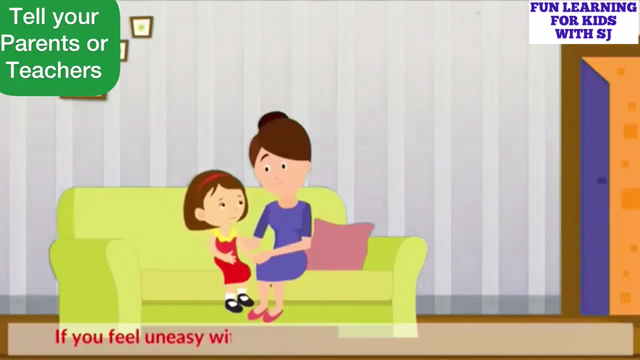 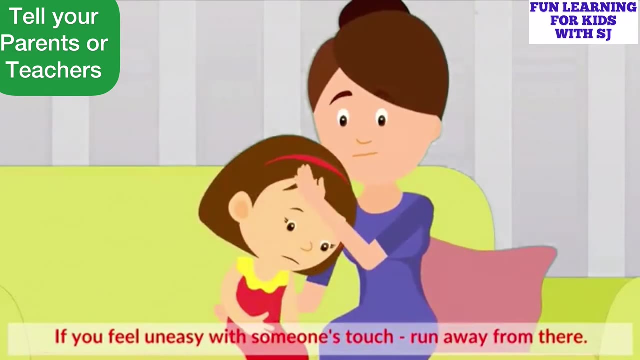 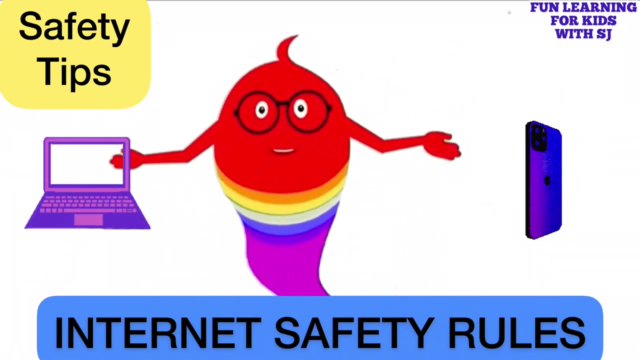 if someone touches you and tells you not to tell anyone. if you feel uneasy with someone's touch, run away from there and tell your parents or teachers about it. here are some safety tips to remember when you are using the internet. always remember the five smart rules, and the best way to get rid of them is to use the internet. 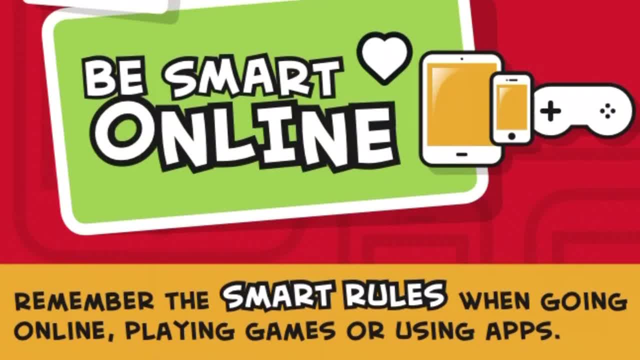 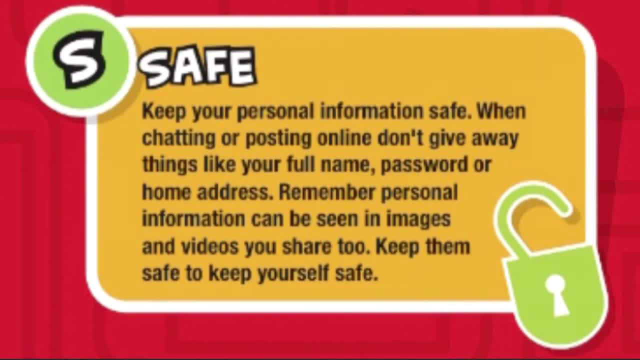 always remember the five smart rules, and the best way to get rid of them is to use the internet when going online playing games or using apps when going online playing games or using apps when going online playing games or using apps s for safe. keep safe by being careful. 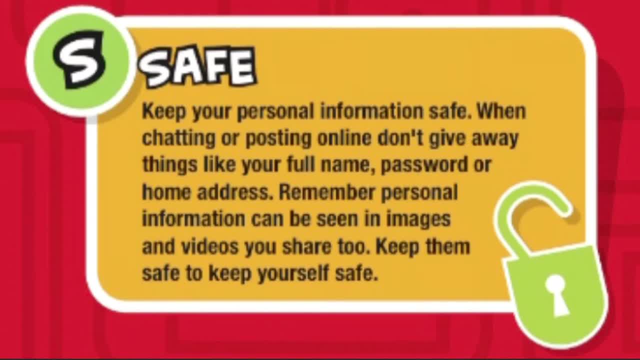 s for safe. keep safe by being careful. s for safe. keep safe by being careful not to give out personal information, not to give out personal information, not to give out personal information such as your full name email address, such as your full name email address, such as your full name email address, phone number, home address, photos or 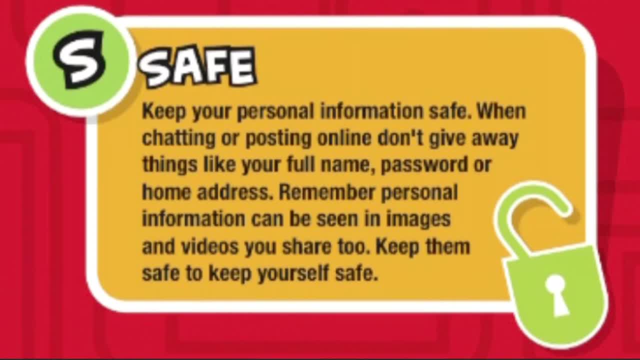 phone number, home address photos or phone number, home address, photos or school name to people you are chatting, school name to people you are chatting school name to people you are chatting with online with online, with online. m for meet meeting someone you have. m for meet meeting someone you have. 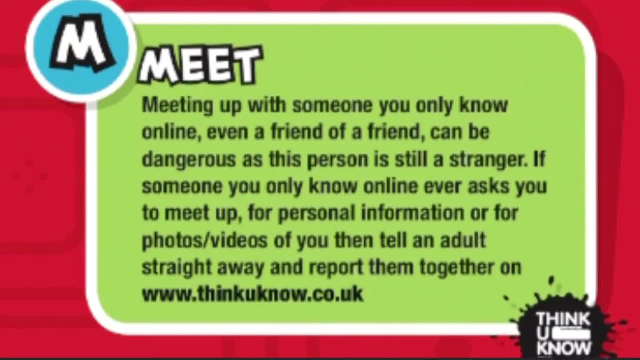 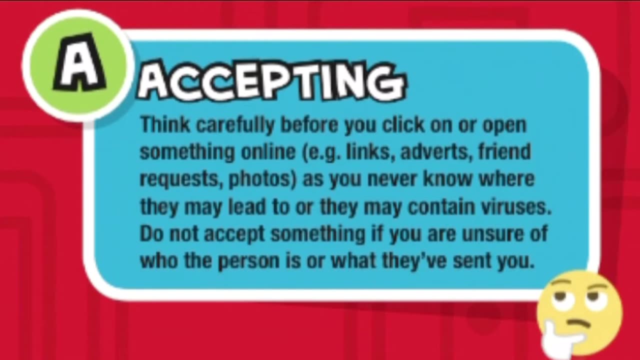 only been in touch with online can be dangerous. only do so with your parents permission and even then, only when they can be present. a for accepting. accepting emails or opening files, pictures or texts from people you don't know or trust can lead to problems they may contain. 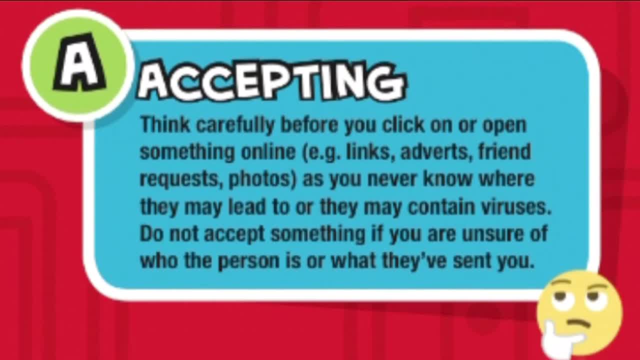 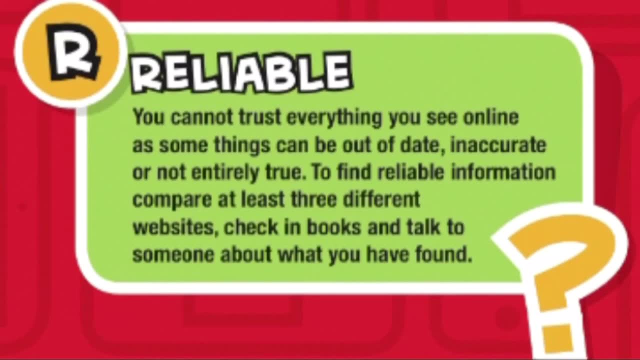 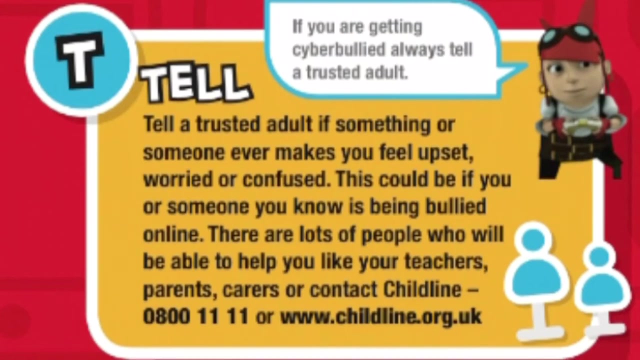 viruses or nasty messages. r for reliable. information you find on the internet may not be true or someone online may be lying about who they are. make sure you check information before you believe it. t for tell, tell your parents or a trusted adult if someone or something makes you. 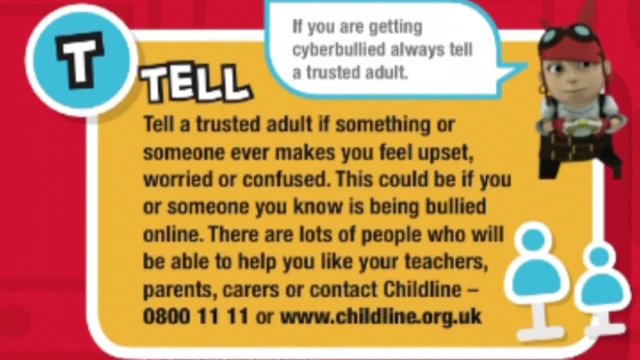 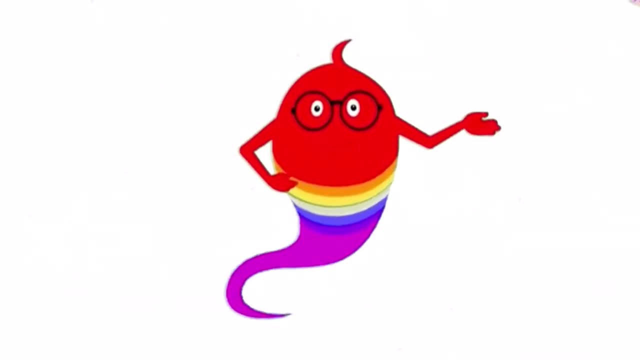 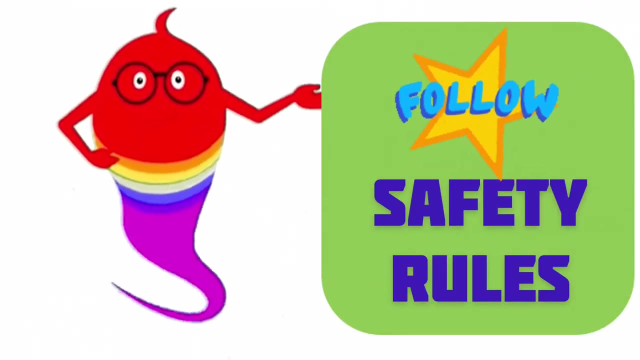 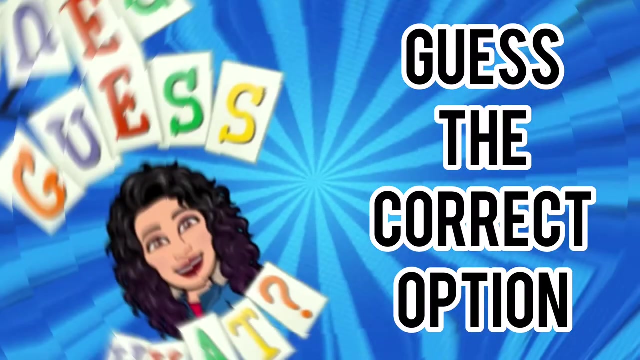 feel uncomfortable or worried or if you or someone you know is being bullied online friends, remember life is very precious and you should take care of it. always follow safety rules and be smart. be safe. it's game time. in this game, you will get three options and you have to select the correct answer. 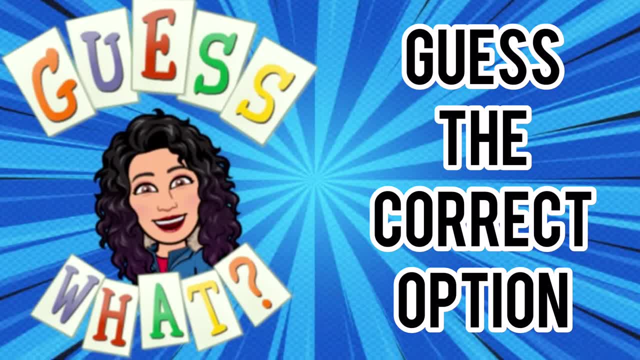 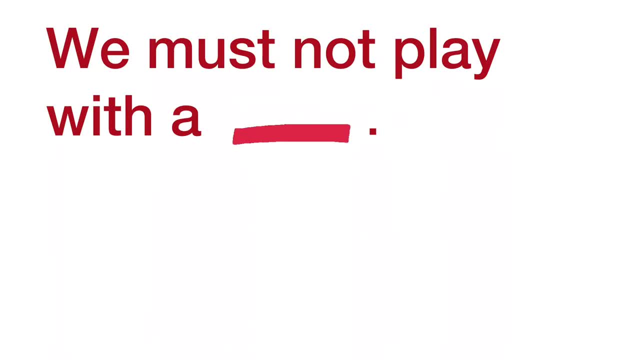 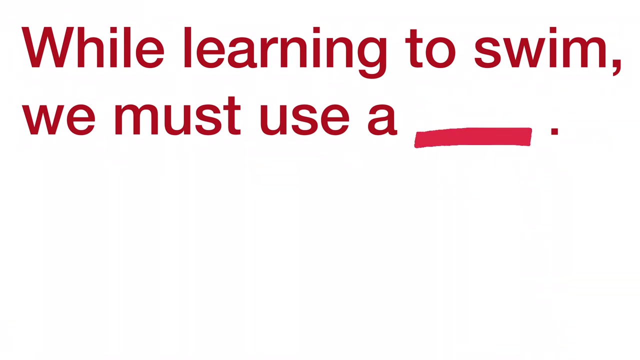 you will get five seconds to guess the answer. i hope you remember all the safety rules. come on, let's start. here is the first one: we must not play with a dash ball toy knife- yes, you're right. the answer is yes, you're right- is knife. we must not play with a knife while learning to swim. we must use a dash blade. 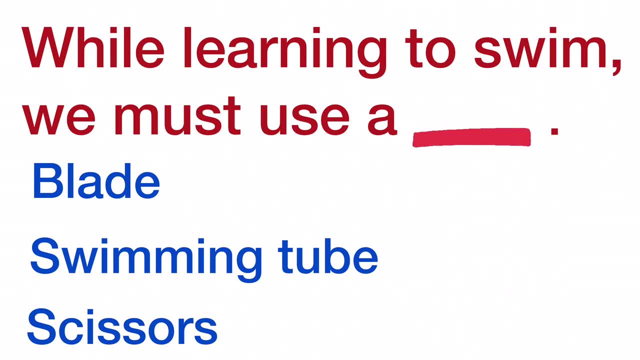 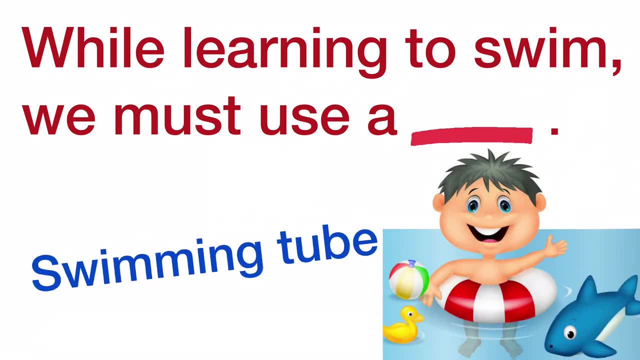 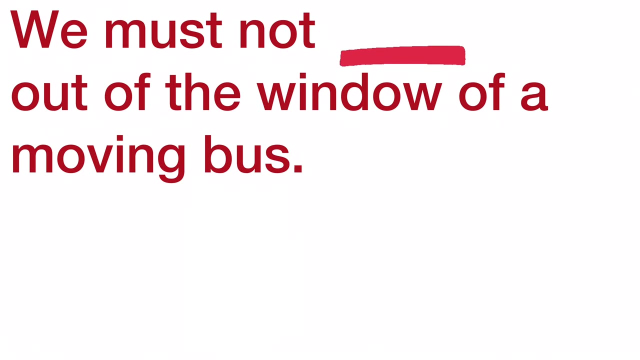 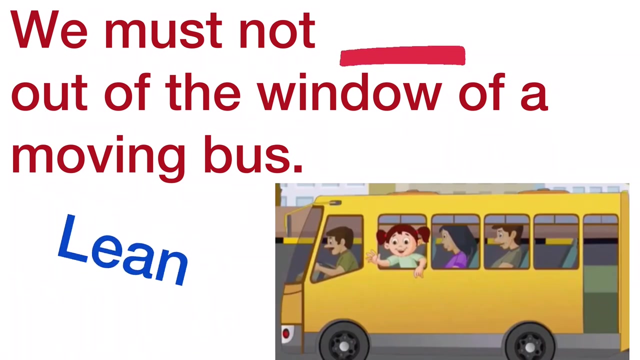 swimming tube scissors- excellent. the answer is swimming tube. we must use a swimming tube while learning to swim. we must not dash out of the window of a moving bus. lean, see both good job. answer is lean. we must not lean out of the window of a moving bus. 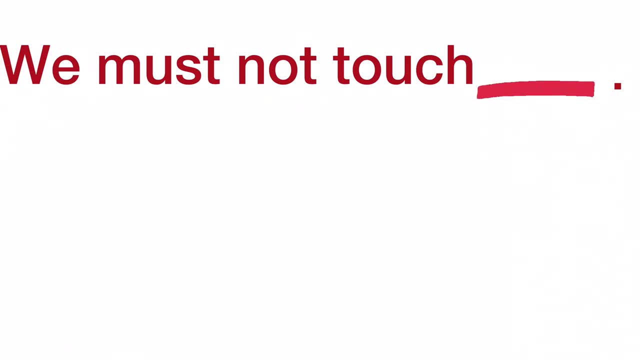 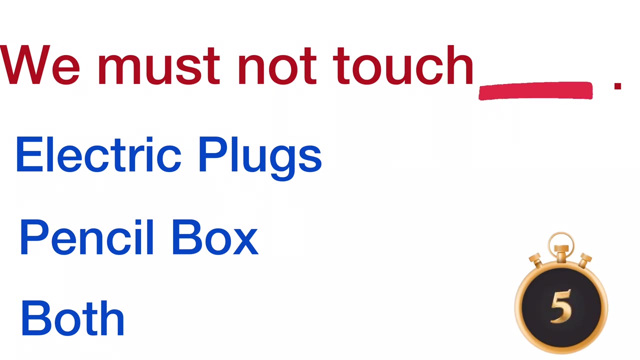 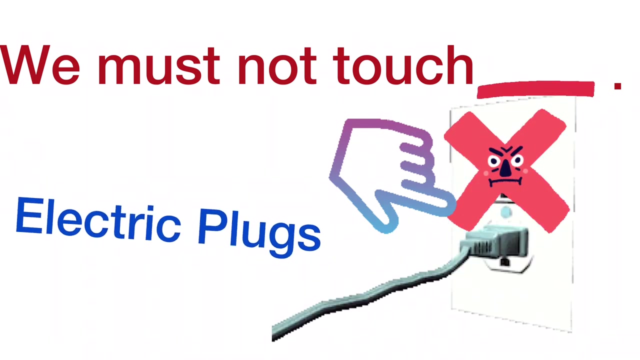 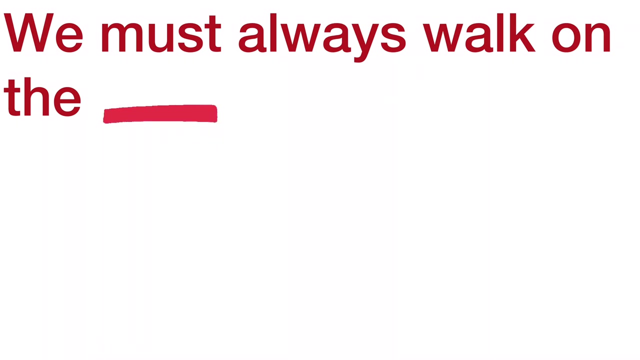 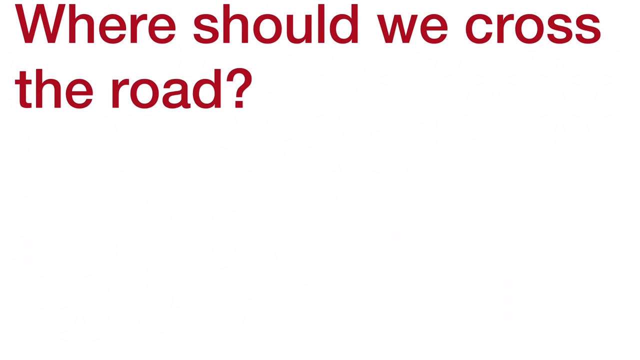 we must not touch dash. electric plugs, pencil box, both- fantastic, the answer is: electric plugs. we must not touch electric plugs. we must always walk on the dash footpath. road rocks- excellent, the answer is footpath. we must always walk on the footpath. where should we cross the road? railway crossing, zebra crossing, both.